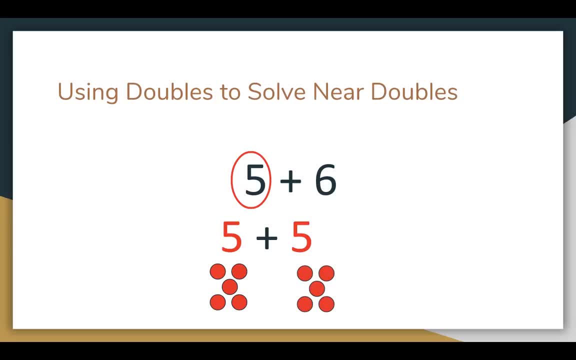 Is 10.. So if I'm doing 1 more because in order to get to 6, I need to add 1 more to 5.. So 5 plus 5 plus 1 more is 10.. In my mind I'm thinking that if 5 plus 5 is 10, I need 1 more to get to that 6.. 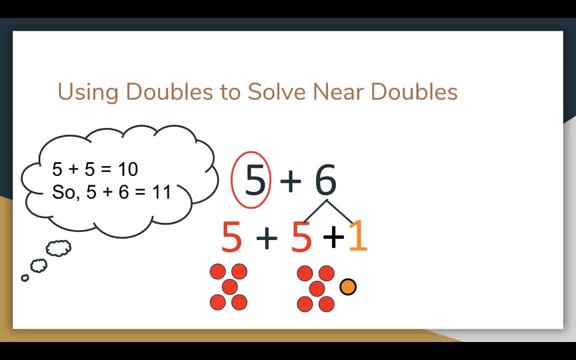 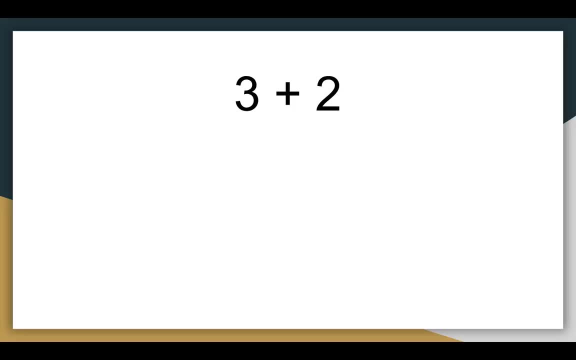 So 5 plus 6 equals 11.. Let's look at another example: 3 plus 2.. So, again to do my adding with near-doubles, I'm going to find my smaller number. Looking at 3 and 2,, I know that 2 is my smaller number. 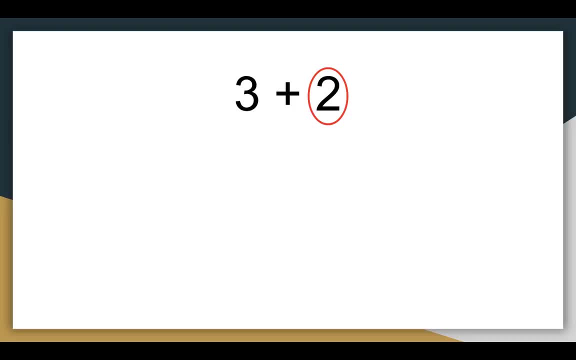 So think about which doubles fact I would make to help me solve 3 plus 2.. You're right, It's 2 plus 2.. If I choose that number, a doubles fact would mean both numbers I'm adding are the same number. 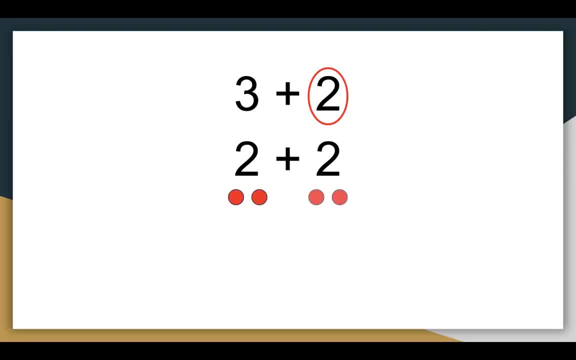 So, thinking about this, I know that 2 plus 2 is 4, but I'm not adding 2 plus 2.. I'm adding 2 plus 3.. I know that 3 is just 1 more than 2.. 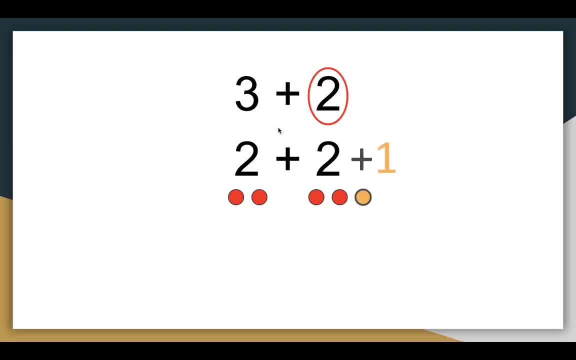 So all I have to do to figure that out is add 1 more. So in my brain I'm thinking 2 plus 2 is 4.. I'm 1 away, so I just need to add more. So if 2 plus 2 is 4, so then 3 plus 2 is 5.. 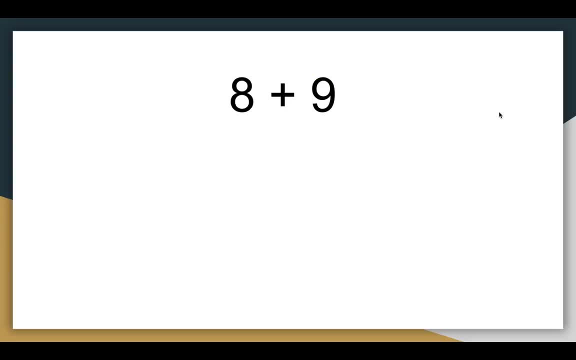 I just have to add 1 more. So I'm not adding 2 plus 2.. I'm adding 2 plus 3.. So I'm not adding. 2 plus 2 is 4.. one more to that sum. Let's take a look at another example together. So right now, 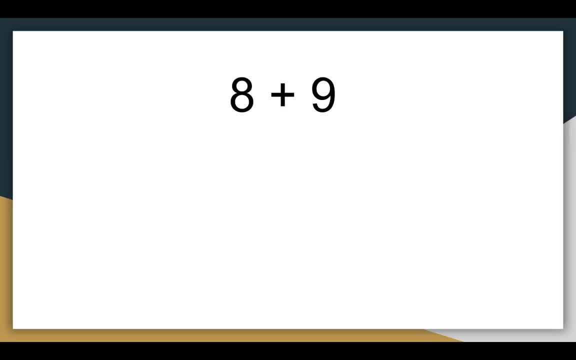 I have 8 plus 9.. So think right now which one would I make. the doubles fact out of 8 is the smaller number, so I'm going to make my doubles fact from my 8.. Write down what doubles fact you would use to help you with 8 plus 9.. The 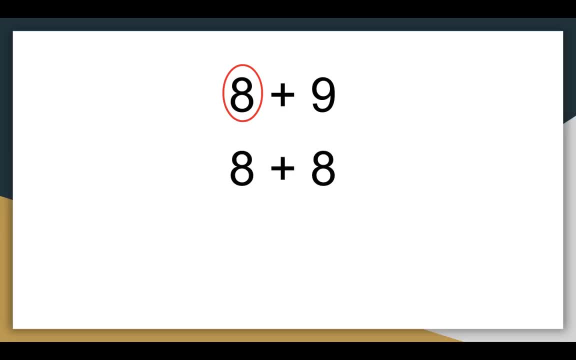 doubles fact you could use would be 8 plus 8.. If I know 8 plus 8, then I can help myself know 8 plus 9.. So 8 plus 8 is 16.. I'm adding 8 plus 9. 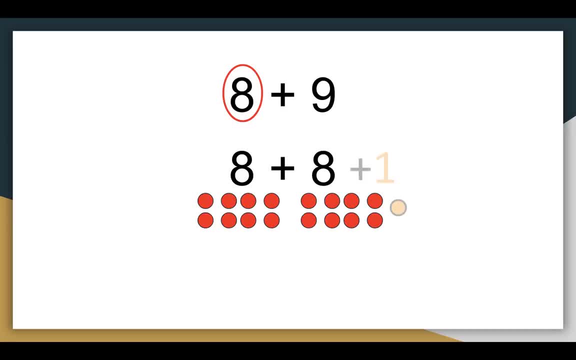 which is only one more than 8 plus 8.. So I add one more to the end: 8 plus 8 is 16 plus one more is 17.. So in my head I'm thinking 8 plus 8 equals 16.. So 8 plus 9 is 17.. It's just one more. 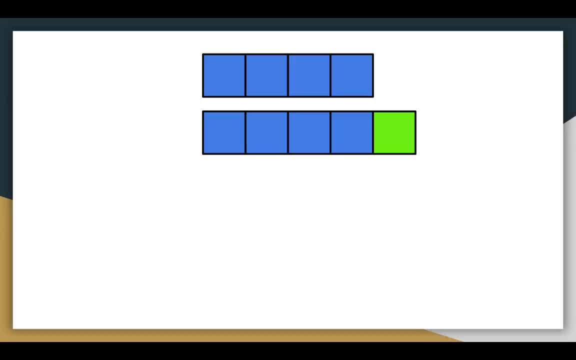 As you're working today, you'll see some examples of problems with some cubes. that can help you as well. So the different colors of cubes can help give you hints on what doubles fact to use as well. If I look at this set of cubes, I see that there are four cubes on the top and they're all. 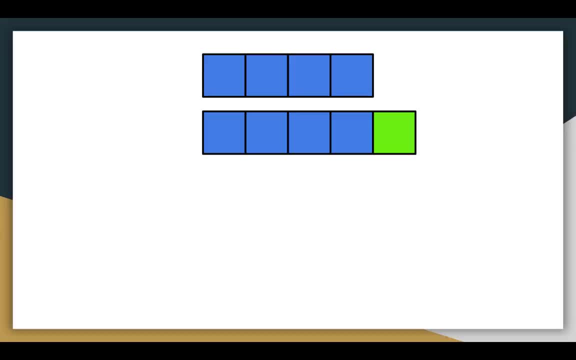 blue, And I see that there are five cubes on the bottom, four of which are blue and one is green. So looking at this, I can see where my doubles fact would be. The blue ones make 4 plus 4.. So, thinking in my head, I know, 4 plus 4 equals 16.. So I'm going to look at this set of cubes and 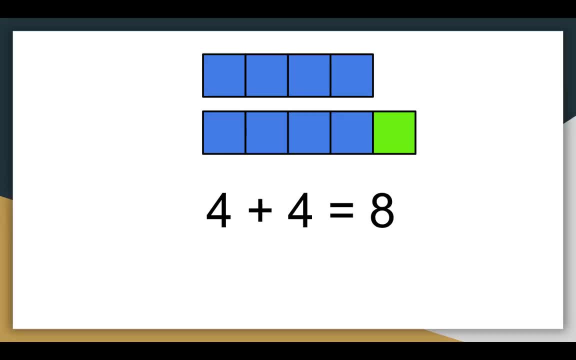 see where my doubles fact would be. The blue ones make: 4 plus 4 is 8.. I only have one more than that, So 4 plus 5 equals 9.. This is the same thinking. It's just using a different visual. 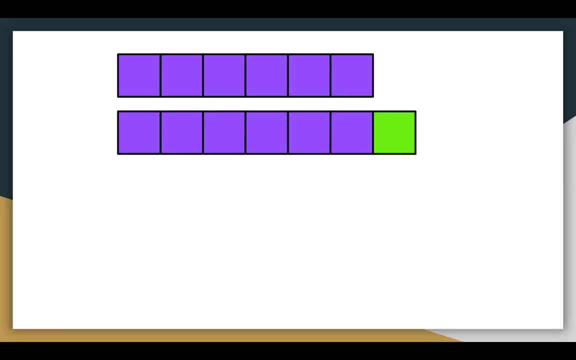 representation. Take a look at one more example. Look at the purple cubes for your doubles fact and then the green one to help you make your new equation. What doubles fact would you use to help yourself solve this? You can pause the video now and write down your doubles fact. 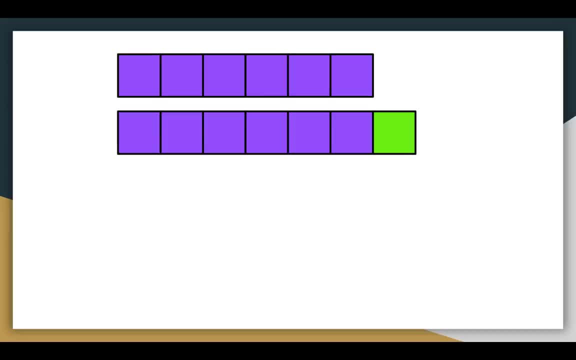 Now that you've written your doubles fact down, we're going to do it together. I can see that there are 1,, 2,, 3,, 4,, 5, 6 purple cubes on the top and 1,, 2,, 3,, 4,, 5, 6 purple cubes on the bottom, So doubles fact.